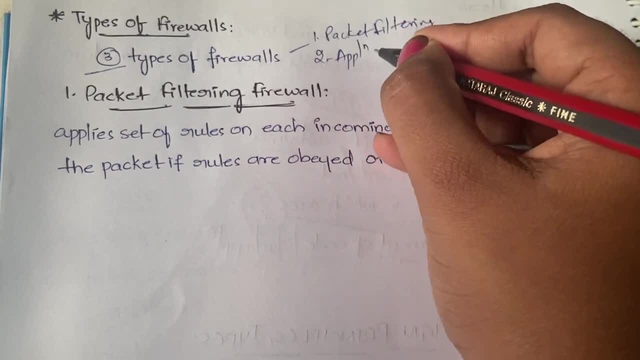 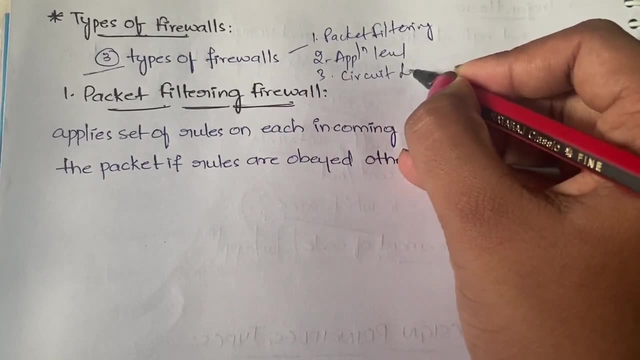 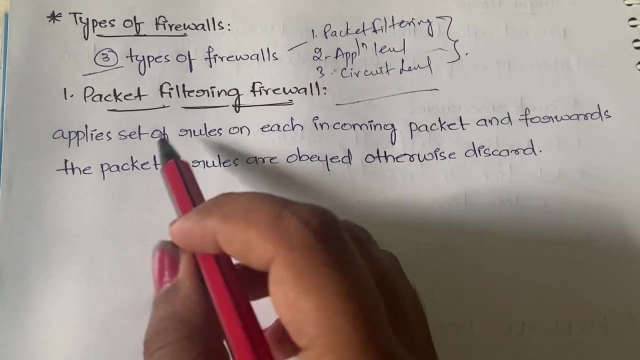 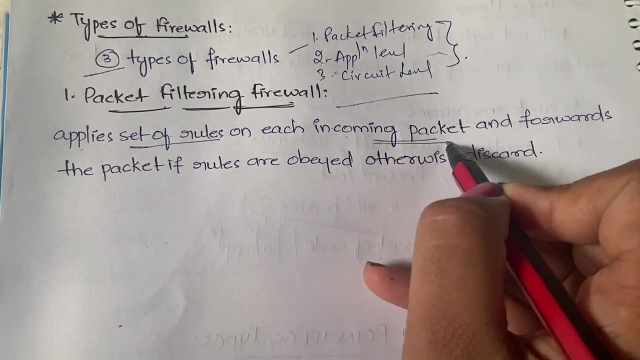 And the second one is application level And the third one is circuit level. Okay, application level gateways and circuit level gateways. We have three types of firewalls. Let us see about each of them now. So in packet filtering firewall, what happens is it will apply some set of rules on each incoming packet. Packet is nothing but data. Data is coming in form of packet. That's all you have learned in computer. 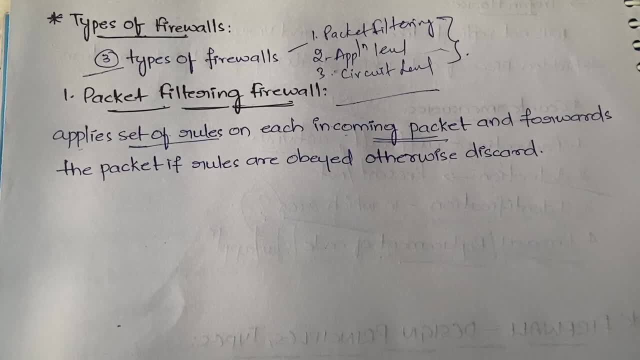 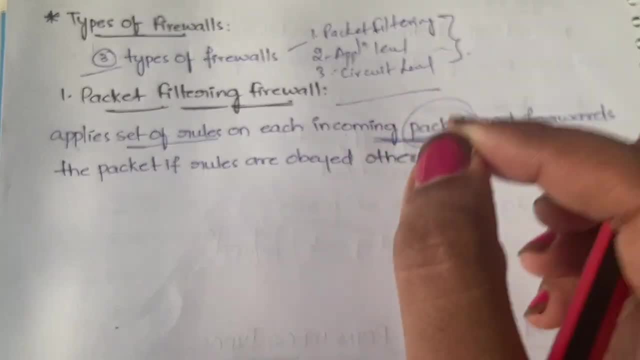 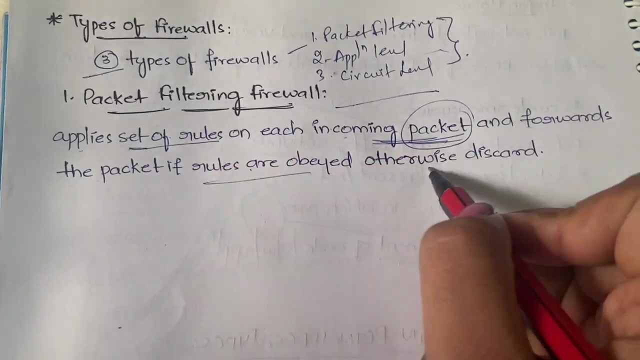 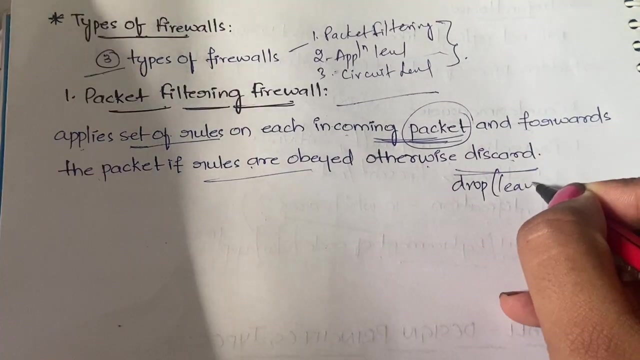 networks. right, What a packet is? frame, datagram and all. So, basically, data is termed as a packet. on each and every incoming packet, you are applying some set of predefined rules And you are forwarding the packet if the rules are obeyed. Otherwise, the packet is discarded. discarded in the sense you will drop it. So you will drop, drop, or you can say you will leave it there itself. you will not forward the packet further in the network. Okay, so it will basically. 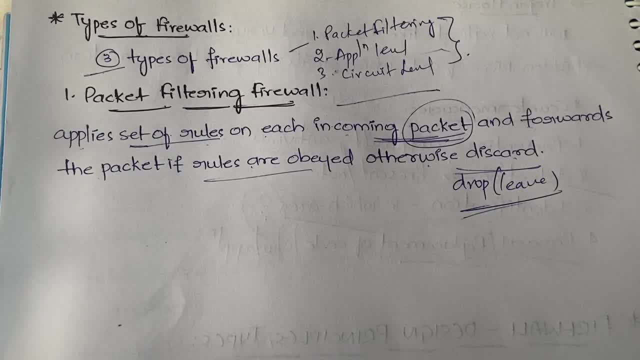 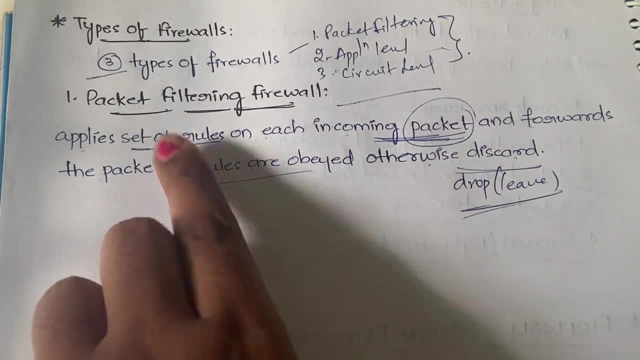 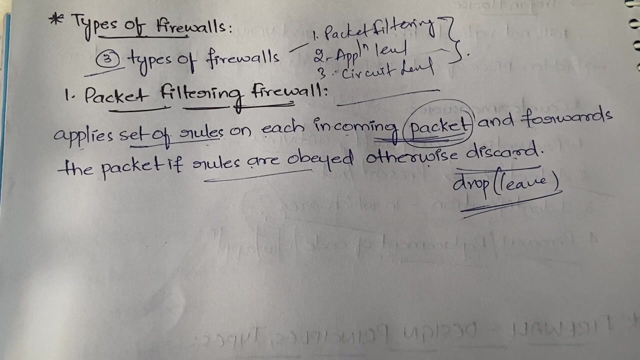 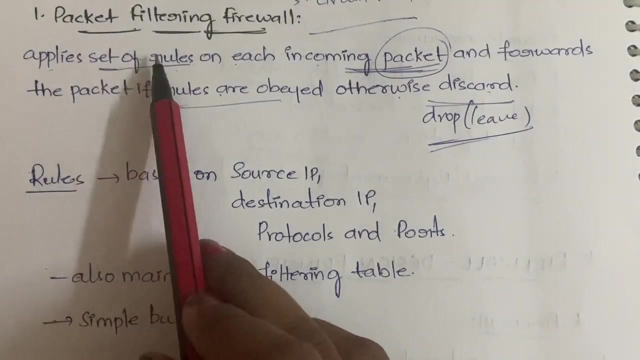 apply some set of predefined rules on each and every incoming packet into the traffic, And if that packet is obeying these rules, these predefined rules, then the packet is forwarded. If not, the packet is discarded, which is nothing. but the packet is dropped then, and there itself Got it. This is about packet filtering, And we have some more. I'll tell you these rules. that is we are. we are saying that, based on rules, we are deciding that whether the packet should be forwarded or discarded, right. So this is about packet filtering, And we have some more. I'll tell you these rules. that is we are. we are saying that, based on rules, we are deciding that whether the packet should be forwarded or discarded, right. So this is about packet filtering, And we have some more. I'll tell you these rules. that is we are. we are saying that, based on rules, we are deciding that whether the packet should be forwarded or discarded, right. So this is about packet filtering, And we have some more. I'll tell you these rules. that is we are. we are. 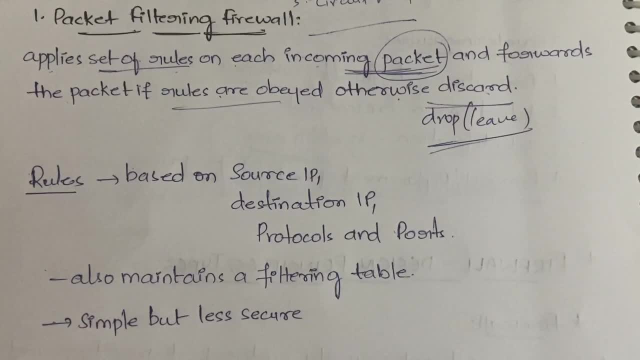 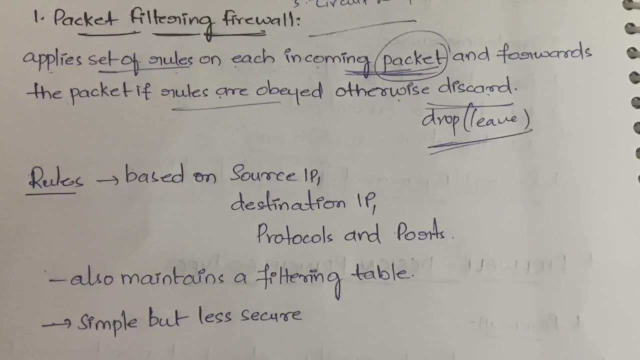 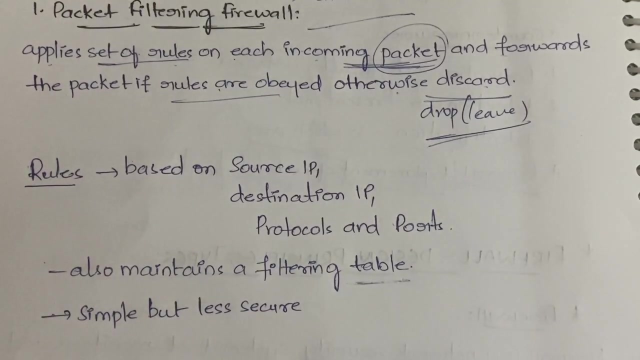 those rules will be based on the source IP address, the destination IP address, the protocols used and the port numbers used. So, based on all these things, rules will be generated- Got it. Next, it will also maintain a filtering table. This packet filtering firewall will maintain a filtering table. This filtering table only will decide whether the packet should be forwarded or discarded. Okay, it will decide, Got it. 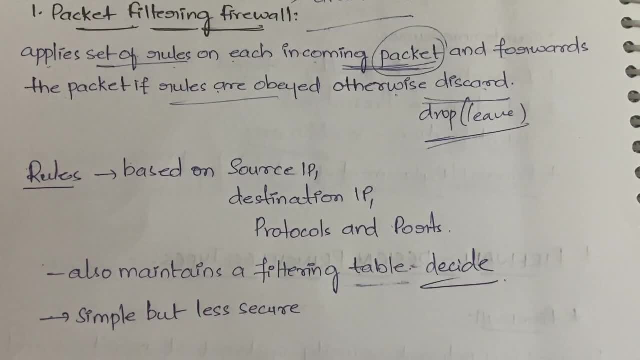 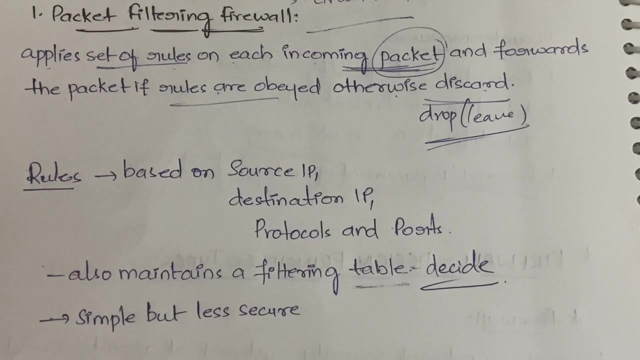 next, it is very simple, but it is also very less secured, since it is simple. if it is simple, obviously security will be less. right, it can be easily known to the attacker. okay, this is about packet filtering: simple. each and every packet is observed and each and every packet is checked. 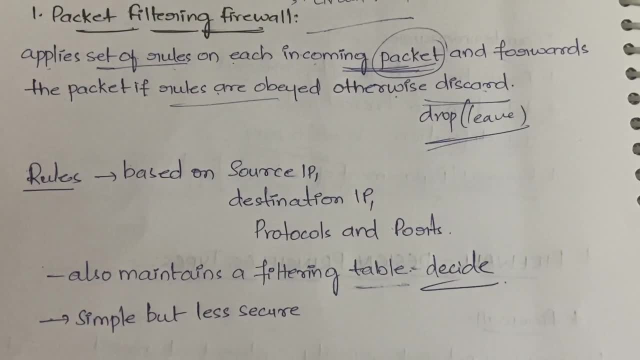 some rules will be applied. it will check whether the rules are obeyed or not. if the packet is obeying the rule, the packet will be forwarded. if the packet is not obeying the rule, the packet will be discarded. got it. next comes the application level gateway firewall. okay, so 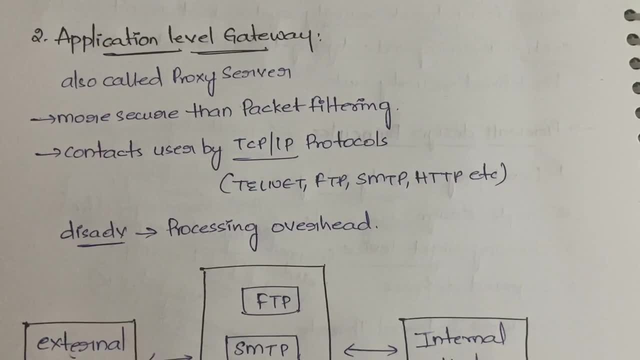 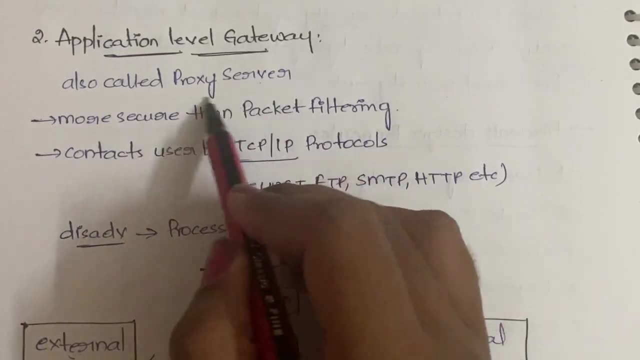 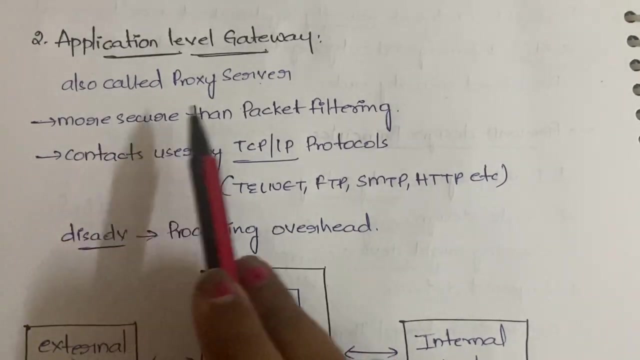 this is the second type. so in application level gateway, what happens is simple. before that i'll tell you. it has also other name, which is nothing but the proxy server. it is also called as the proxy server. you know what? a what word? proxy means right, and it is more secured than the. 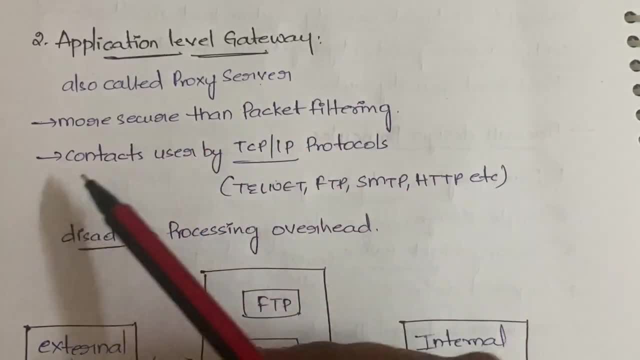 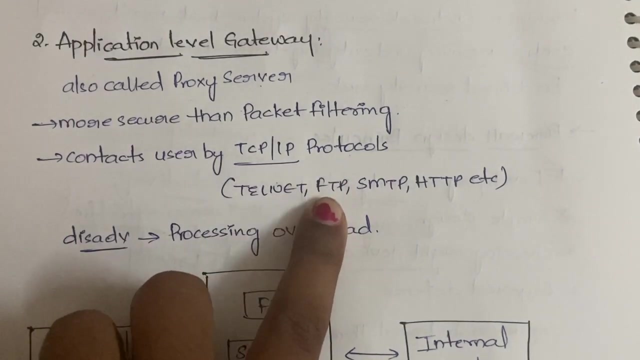 previous one that is more secured in the packet filtering one, and it will contact the user by using tcp ip protocols. any one of the tcp ip protocol it will use and through that protocol it will communicate with the user. those protocols could be telnet, ftp, file transfer protocol, smtp, simple. 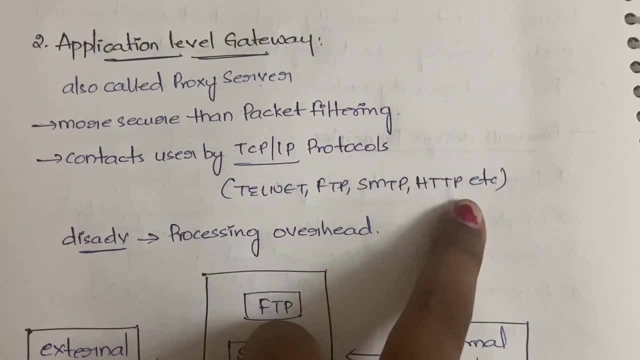 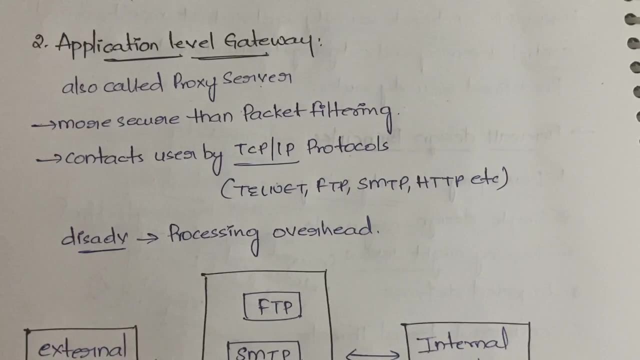 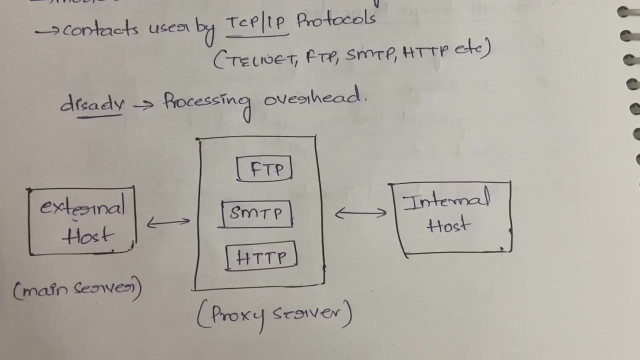 mail transfer protocol, http hypertext transfer protocol, so any of these protocols can be used and communicated with the user. and here, what is the disadvantage in this method is there will be processing overhead. why processing overhead? i'll tell you. so the main piece is the signal test. you get the type and it's function for the domino, so you get. 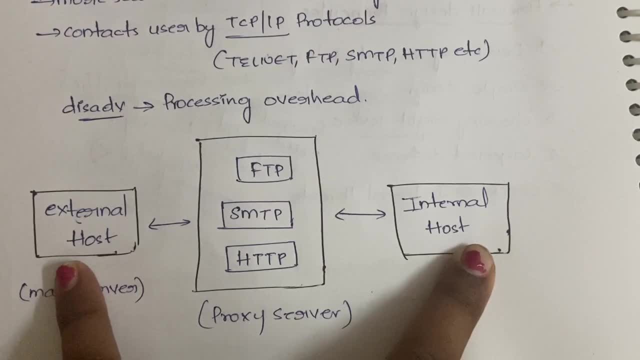 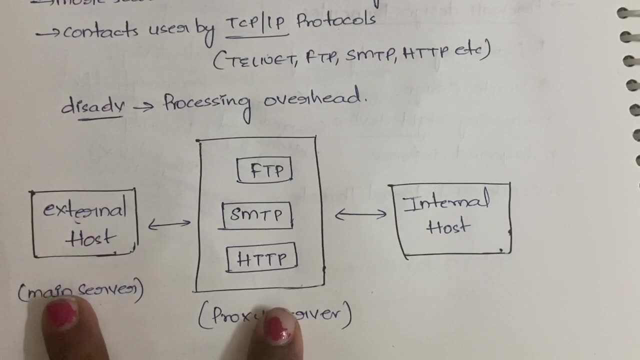 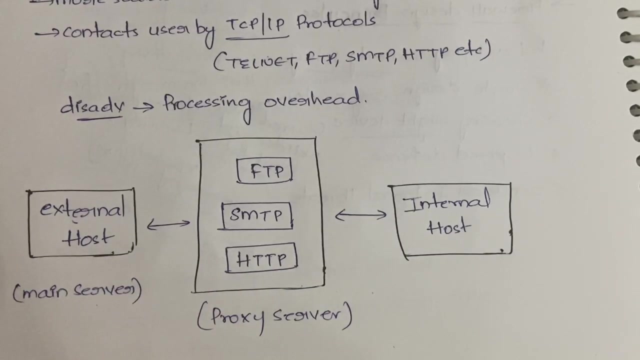 a signal that any form or object would be functioningiage at any point. so for eей, Pork and llama. haha. so at the surface level it's upstairs. we have a call, null user network, call name remember. and when we say, can you hear my voiceston, throat is r quiet clear. can you hear me? 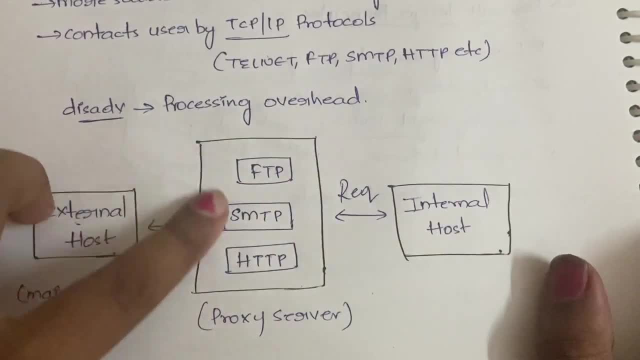 okay, here we have the tied screen forward for the data currently. so this is our list of the softwares happening here, and it organization is already capable. so it's important to plot out programs for that fact before we move moving forward. so what will be happening here? we will use a Bazin. 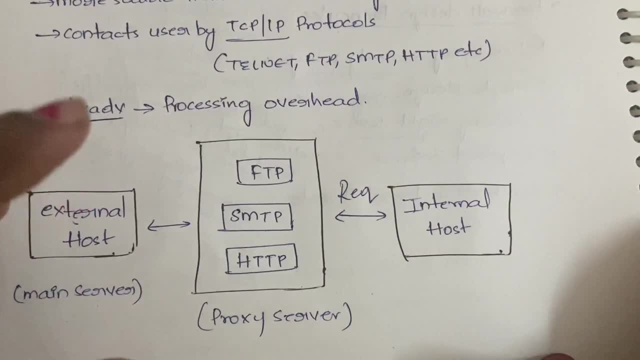 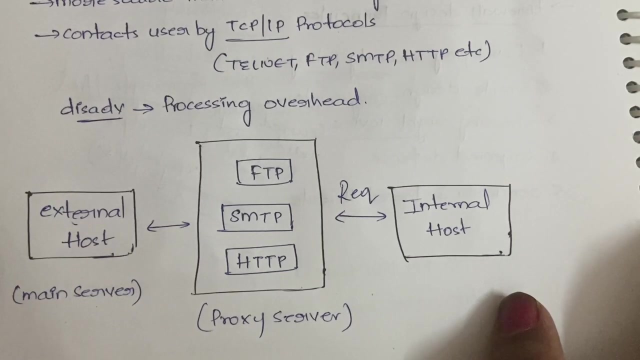 HTTP, as we, as we have discussed here. so the internal host will be sending the request to the proxy server. and what proxy server is doing now? it will check for the authentication of the internal host. so if, if, whether the internal host is an authenticated person or not, he is he from third party or so that it will 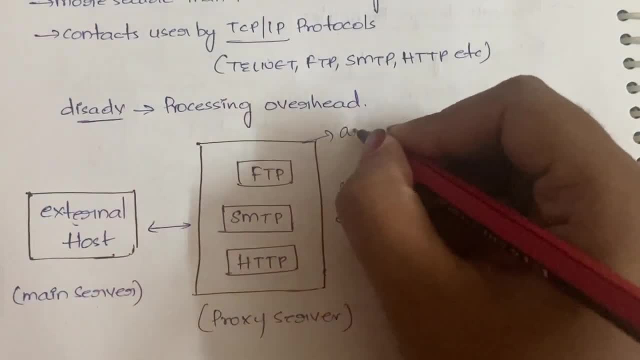 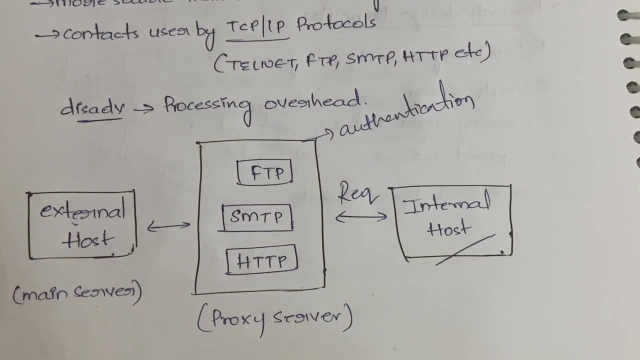 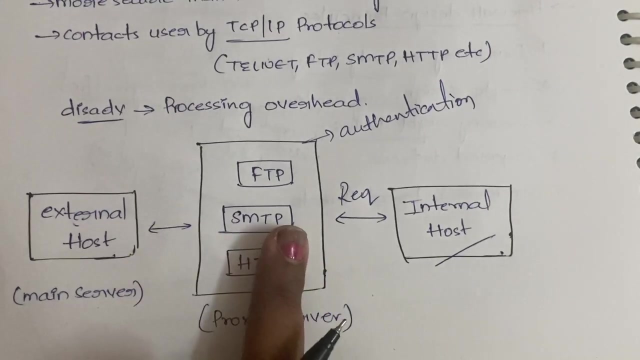 check for the authentication. it will check for the authentication of the internal host. okay, once it checks the authentication, if it is authenticated, if it is good, if it is a reliable one, then the proxy server will send the same request to the external server. okay, the proxy server will send the same request. 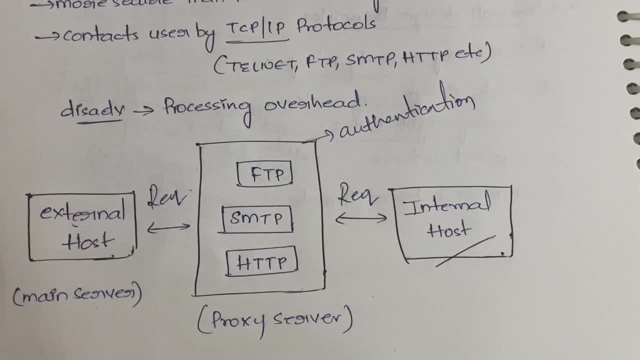 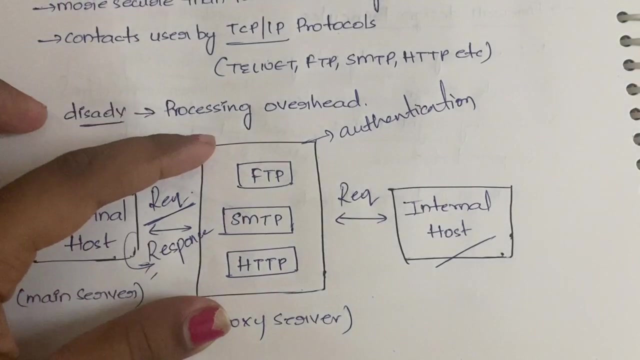 to the external server. now what external server will do? it will send the response to the request. so, whatever request is asked, to that request, a relevant response will be sent to the proxy server first, not directly to the internal host. now what proxy server is doing? it is again checking for authentication of the information, which 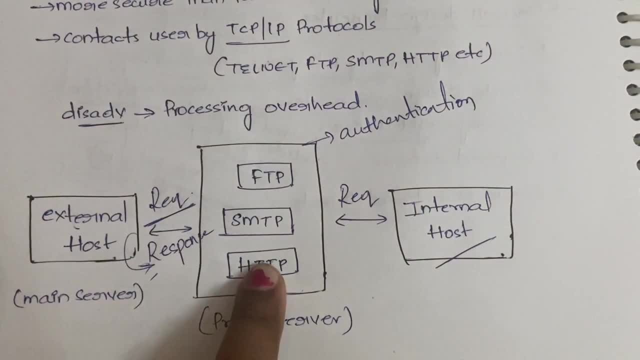 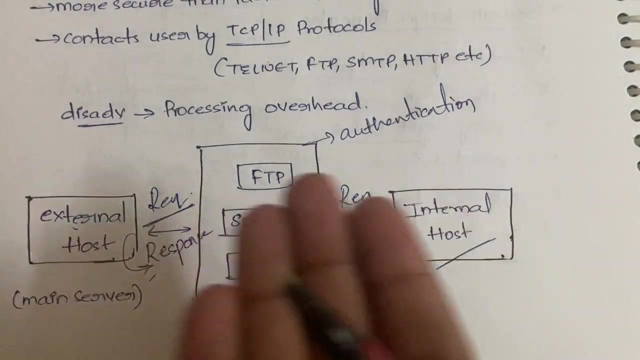 the external host has sent okay. again, once authenticated, the response will be given to the internal host got it? this is the process that happens. but what internal host will feel it feels like it is Directly sending the request to the external host, that is, it is directly sending the request to? 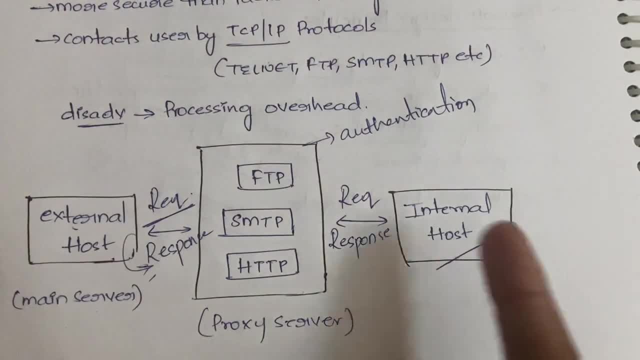 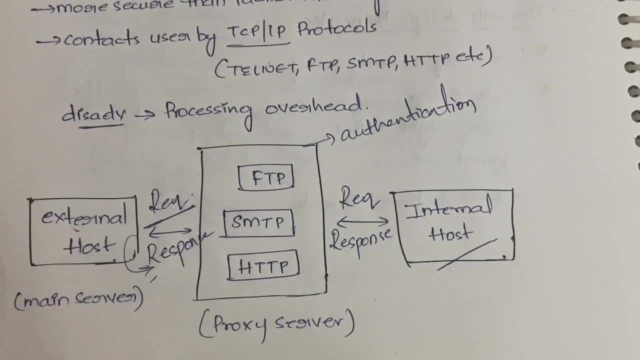 the main server, it will think: but actually the request is going to the proxy server. okay, then the proxy server will check for the authentication and from there it will send to the main server. main server will also give response and that response also is checked by the proxy server whether it is a reliable one or not. once done, then that will be again. 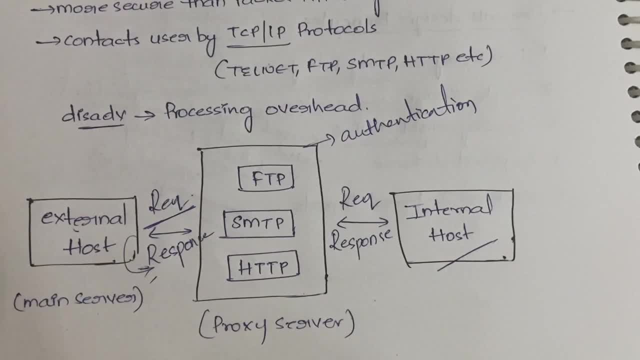 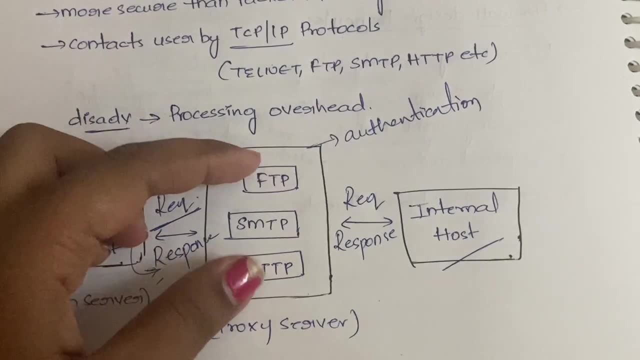 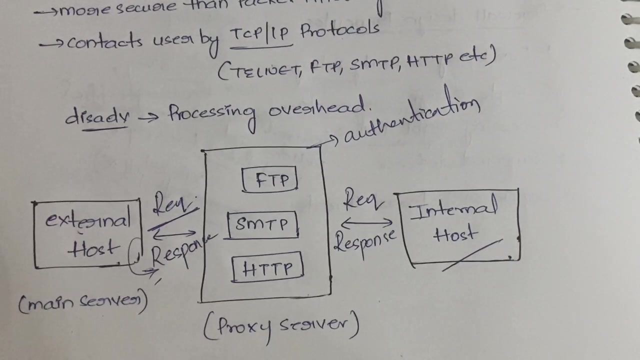 sent to the internal host. this is how communication will happen, and communication between these two things, i mean the internal host and the external host, will happen by any of these protocols based based on the scenario. okay, so this is about application level gateway. now, after this, we have the third one, that is, circuit level gateways. so in circuit level, 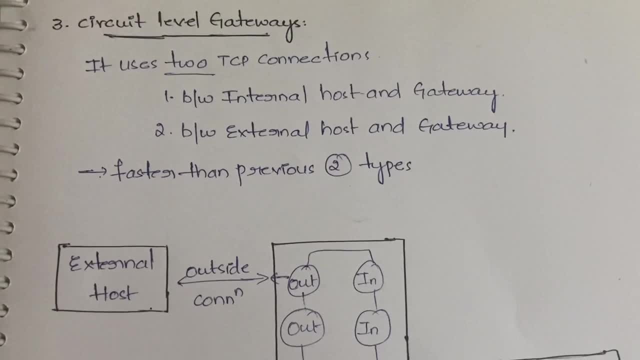 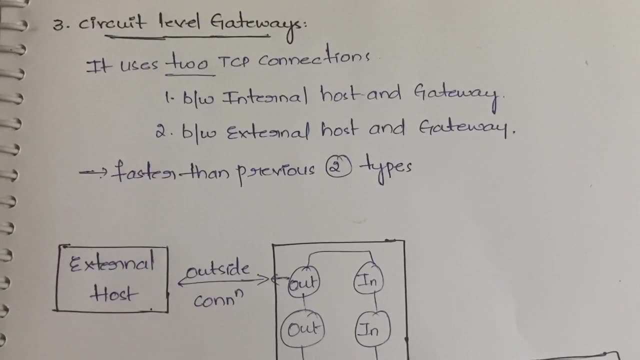 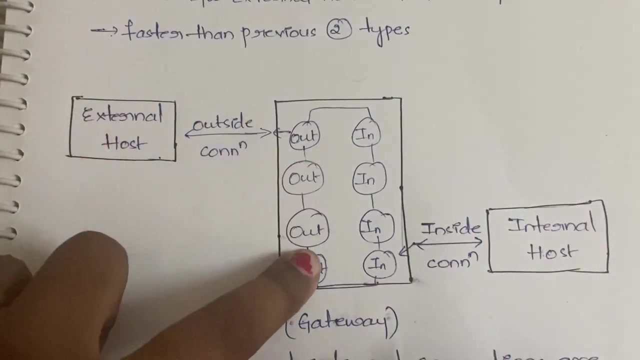 gateways. what will happen again? this is also simple to understand. it basically has two connections. it will also have some external host. it will also have some internal host, but here, instead of proxy server, we are having a gateway. okay, so this is the internal host, external host, and this is the.